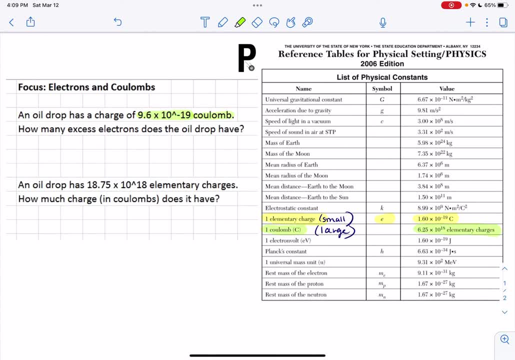 the negative, 19 coulomb. How many excess electrons does the oil drop have? All right, so we are converting from coulombs to electrons or elementary charges. So when we set it up, I'm going to set it up just like we would for dimensional analysis, coulombs, and we need to set it up with a ratio. 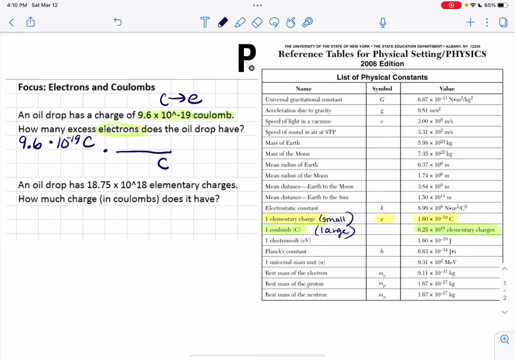 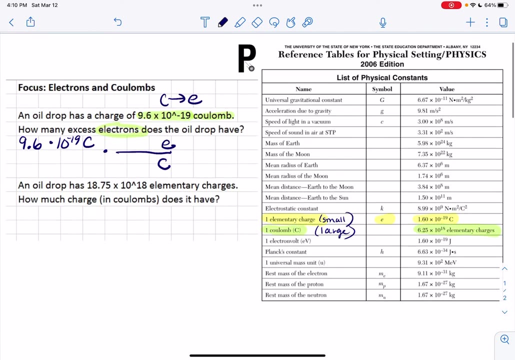 So it doesn't matter which ratio we use, but we have to put coulombs in the denominator and elementary charges. So technically you could use, you know, either elementary charge ratio, the small one or the large ratio. For me personally, I like to put one in the denominator and then use whatever ratio. 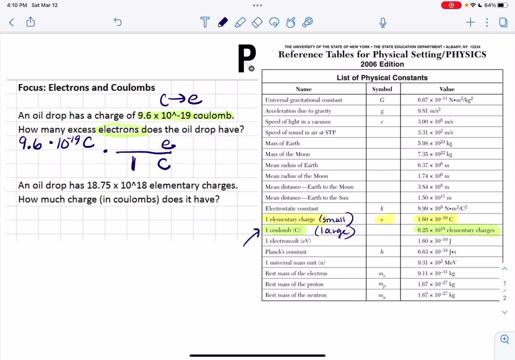 that is. So one coulomb, for instance, this one right here, is 6.25 times 10 to the 18.. So I like setting it up that way, because coulombs I cancel out with coulombs and since it's a one, we just 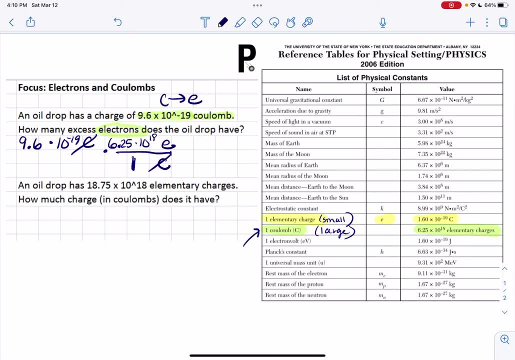 multiply straight across in our calculator And then we get the answer. And I of course, did not bring my calculator over here, so I'll just do it real quick online. and we do it this way. So it's going to be six elementary charges. So I like to 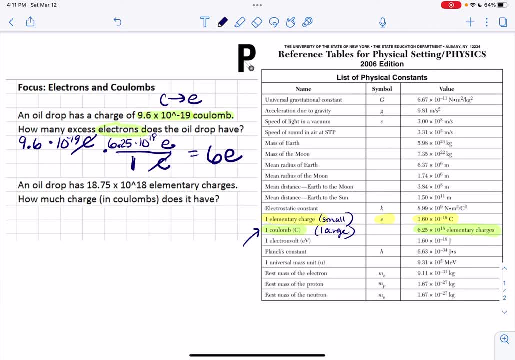 set it up that way. You could put one elementary charge is the same thing as 1.6 times 10 to the negative 19 in the denominator. The only thing is then you would have to put parentheses around the whole thing when you divide. But you can do it. 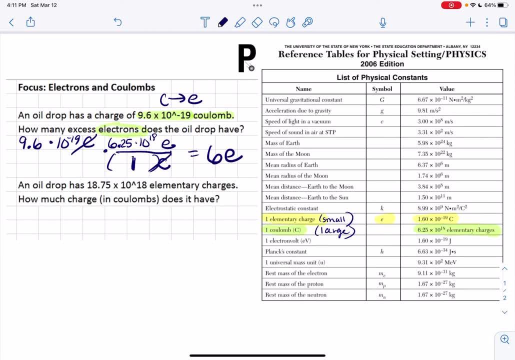 either way. Either way would work. So the same idea with this next one. It says an oil drop has 18.75 times 10 to the 18 elementary charges. How much charge in coulombs does it have? So we are given 18.75e And to set up this: 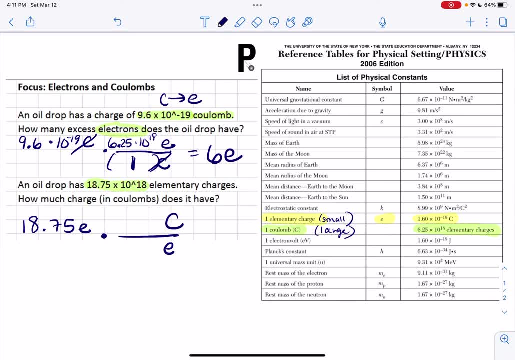 ratio. we have to put e in the denominator and coulombs on top. So again I like to put one in the denominator. and then So again I like to put one in the denominator and coulombs on top. So again, I like to put one in the denominator and 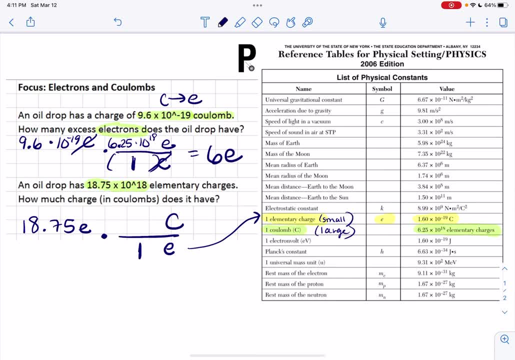 the denominator. So if I do that, that means I need to use this ratio here. So then I get 1.6 times 10 to the negative 19.. So E cancels out. with E we multiply that straight across, And when we 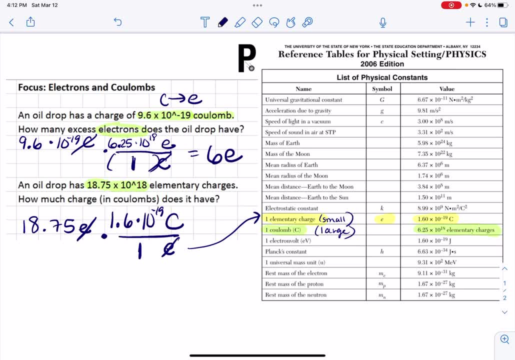 do that again. I'm just going to use my computer real quick And then that gives us our answer in coulombs. So in this case it would be three coulombs. So that's basically how you do it, And 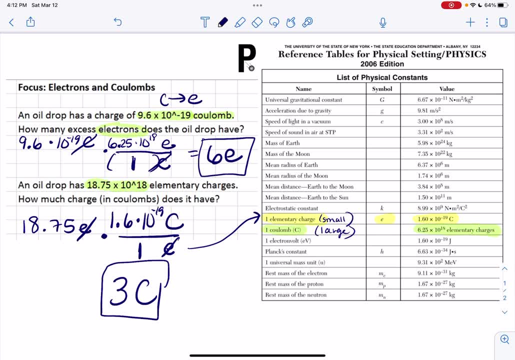 you could use either ratio. you just need to set it up correctly and find a way that works best for you. But the answers for these two is six elementary charges and three coulombs. 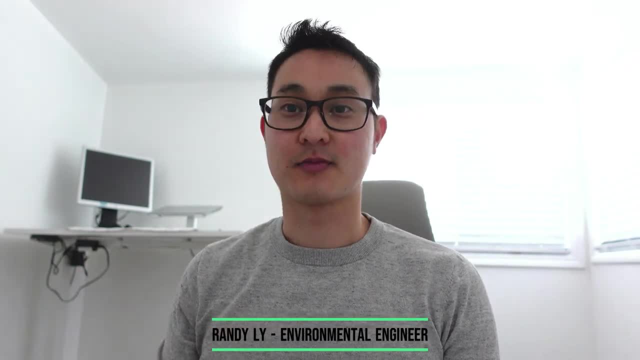 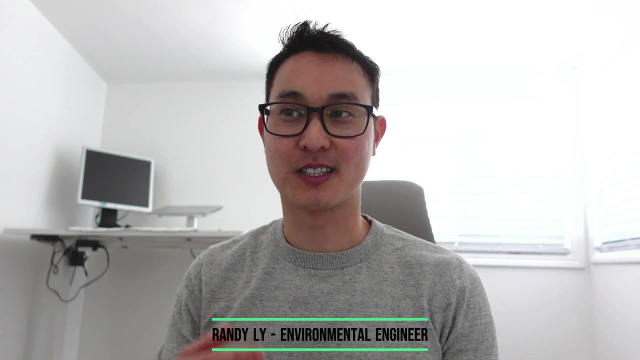 Hey everyone, my name is Randy Lee and I'm an environmental engineer. I've been working in my profession for about five years now, so I can say with some certainty that I have some experience and know something about the environmental engineering field, more so than the average.